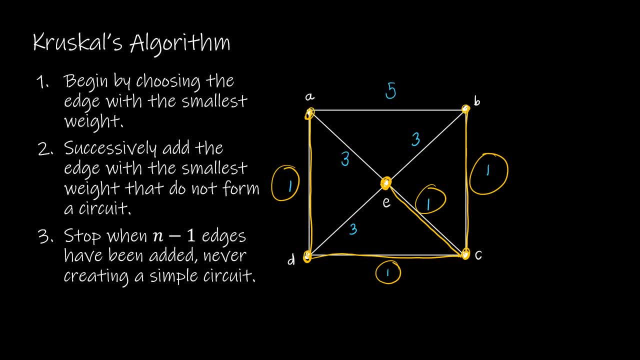 this one. So we can see that I've now connected all of the vertices and I have the least weight because I've chosen all of the vertices with the least weight. So then, my spanning tree, my minimum spanning tree, would go from A to D, from D to C, from C to both E and B. 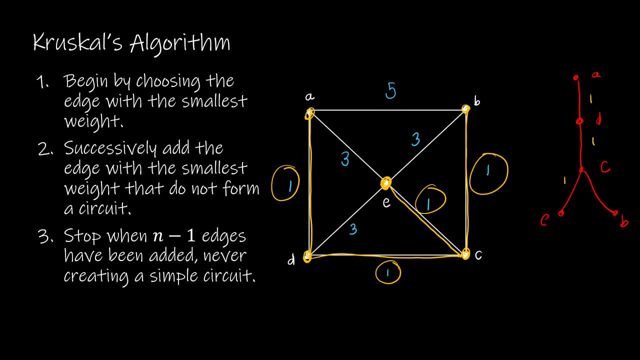 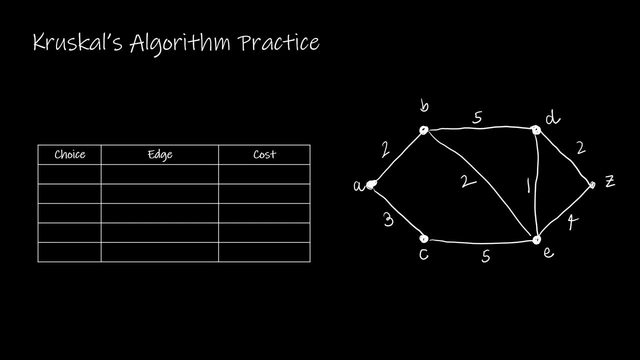 and each weight is 1.. So I have a total weight of 4.. So, looking at our first practice together again, I've created a table for you- and that's mostly for my benefit- so that I can see your choices, but it also gives you a little bit of an idea of what you're going to be doing next. So I'm going. 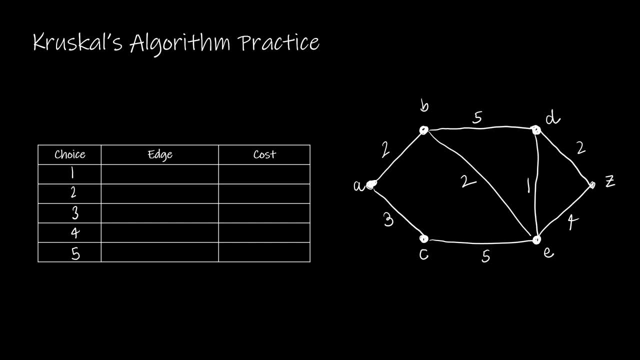 to start by choosing the cheapest weight. Again, I haven't been asked to start at a specific vertex, because with Kruskal's algorithm you're really just going for the cheapest weight first. So my edge here would be D, E with a cost of 1.. Then I'm looking at all of the other costs. on. 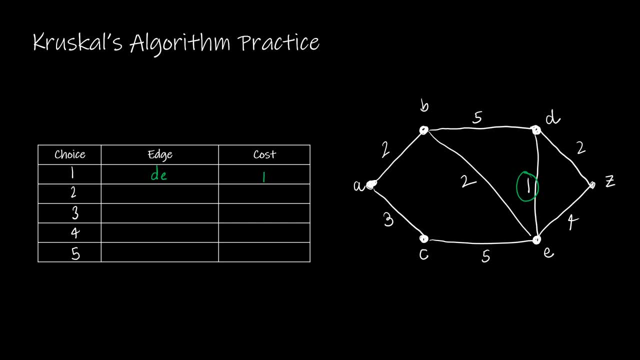 my graph and we can see I have quite a few 2s, So choose a 2.. It doesn't matter which one you choose. I'm going to choose D Z with a cost of 2.. So D Z, cost of 2.. I have some other 2s. I'm going to. 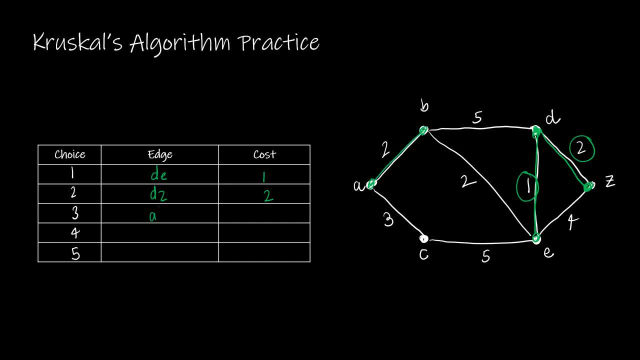 choose A, B with a cost of 2.. And again, I still have another 2, and the only thing I have to worry about is: does it create a circuit? and it doesn't. so I'm going to choose it. So I'm going to choose. 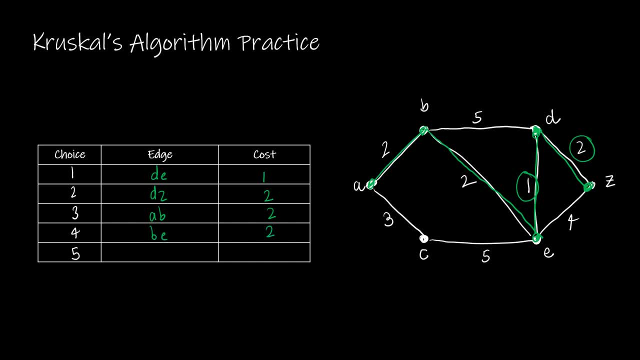 B, E, with a cost of 2.. So again, I'm really just choosing A, B with a cost of 2.. So I'm going to choosing the cheapest cost each and every time. Now I do have some more values on the graph I haven't used yet, but the only vertex I haven't yet visited is C. So really I'm just looking at the. 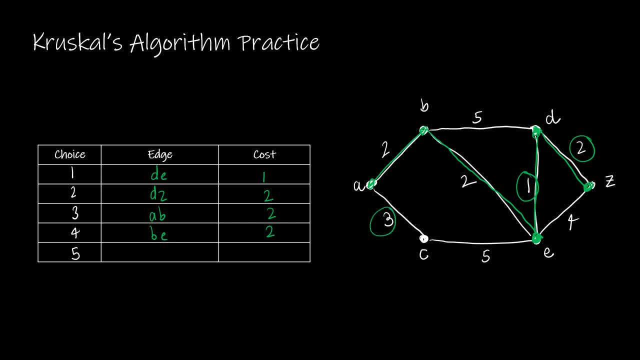 cheapest weight to get to C, which in this case would be 3.. So now I'm going to add AC and that cost is 3.. So again, if I am adding up the total, 1 plus 2 plus 2 plus 2 plus 3 is 10.. That's the. 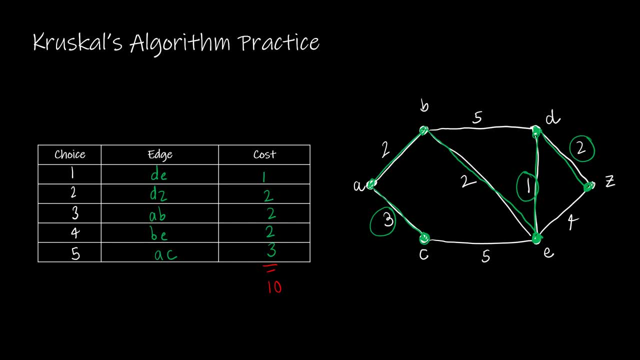 average value of AC. Now, I've already created this with with prim and creating that minimum spanning tree. I would just start with a. a branches off into both B and C. B branches off just down into E, And E to D and D to Z. 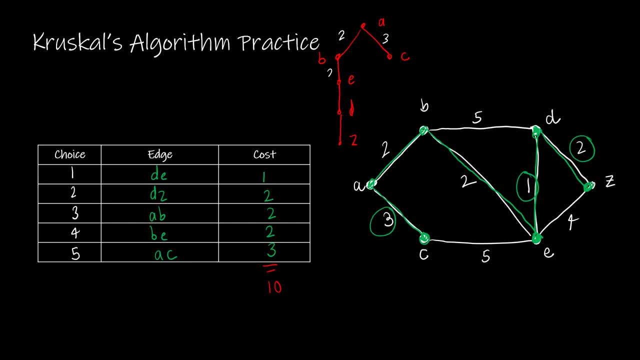 Again, adding those weights, A to B is 2.. e is 2, e to d is 1, and d to z is 2.. So again I've got a total weight of 10, and there is my minimum spanning tree And again you'll notice, it's the same tree that we created using Prim's. 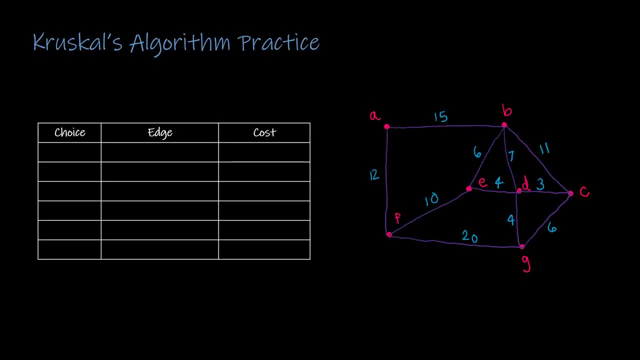 algorithm. Here's a practice for you to do on your own. So if you would press pause, try this question. When you're done, press play to see how you did So. again, my first choice would be whatever the cheapest method is, which in this case would be 3.. So I'm going to add dc, which is 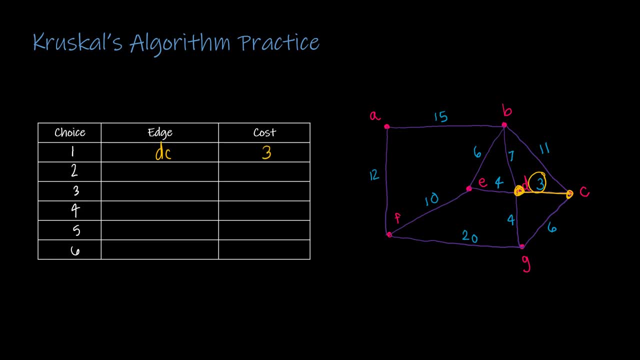 3. From here I'm going to add a 4.. So there are obviously two 4s. I'm going to choose whichever one I want, which for me is dg, with a cost of 4.. And then I'm going to also add de, with a cost of. 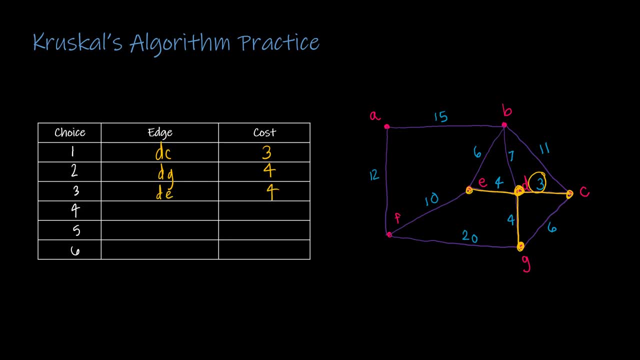 4.. Now, looking at the values on my chart graph, I do have a 6 here, but, as you can see, this 6 isn't going to work because G and C are already part of my minimum spanning tree, So I am going to choose instead this 6, which is E to B. 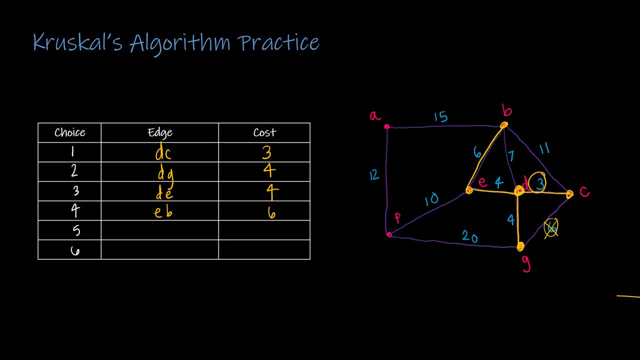 with a cost of 6.. 7 seems to be the next lowest number, but again 7 is not going to work because D and B are both part of my graph. already, Continuing up the ladder, I've got 10,, so I'm. 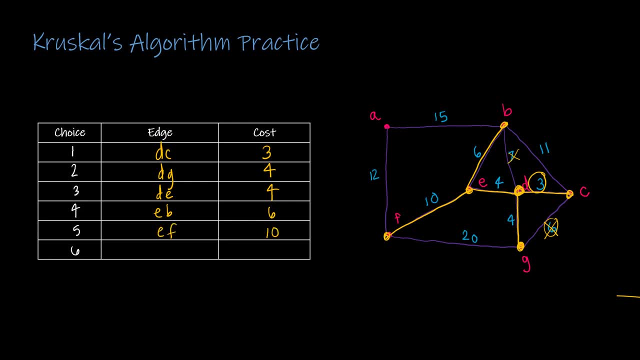 going to use EF, which is 10, and then I'm looking for any way to get to A, because A is the only vertex I have not yet visited, and so the cheapest way there is 12.. So that's AF with a cost of 12..